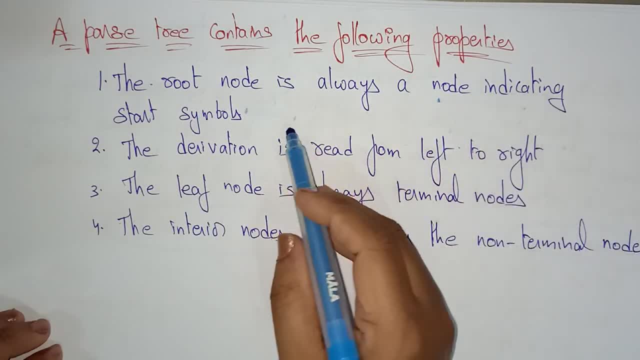 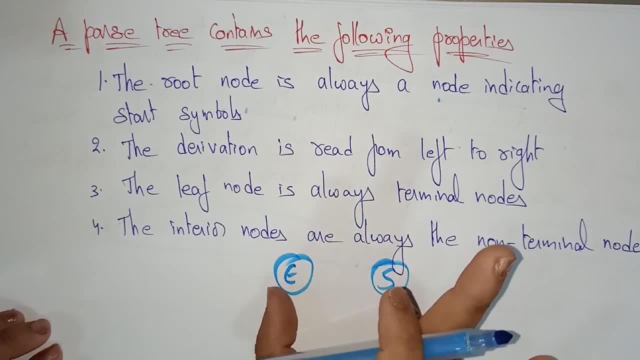 these properties. the root node is always a node indicating a start symbol, so the root node should be a start symbol. either it is a e or a s, whatever it may be, the root node should be a start symbol. that is okay. start start symbol. the derivation is read from: 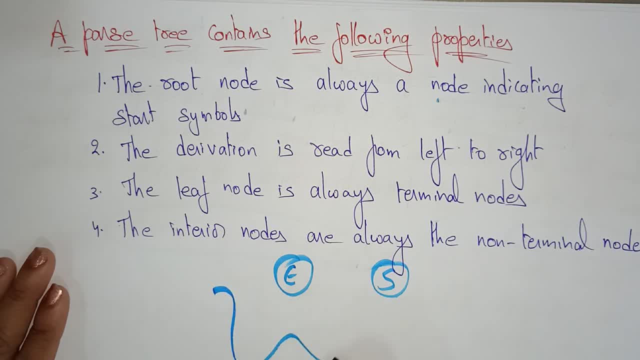 left to right. so we have to read the derivation from left to right. okay, suppose, whatever the tree that is you are representing, you have to start the reading from left to right. so derivation is always read from the left, starts with this node, left side node, and then go and then. 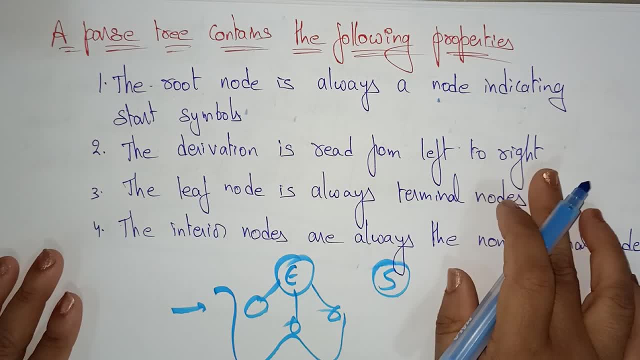 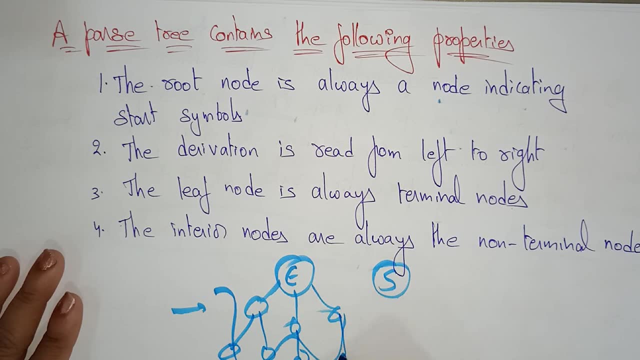 like this: okay, the derivation of is read from left to right. the leaf node is always a terminal node, so remember that, whatever the leaf nodes that are present, okay, these, these are the leaf nodes. whatever you are going to read, whatever you are going to read from left to right, these, 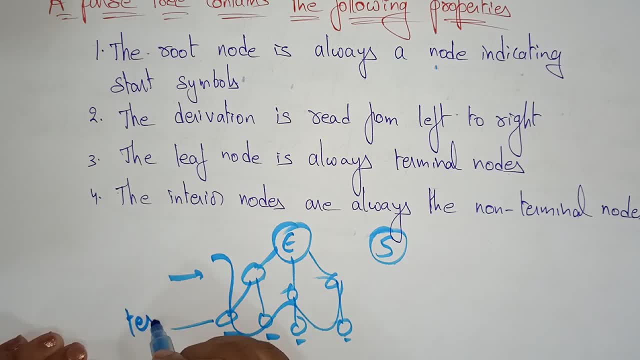 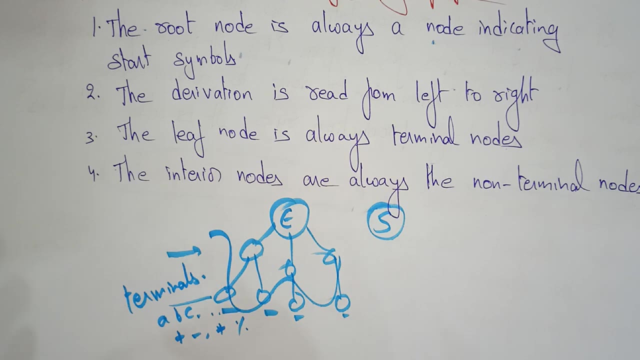 leaf nodes is always a terminals, a terminals may be a, b, c, like that, or plus, minus star divide. so these are all the terminals. okay, other than the capital letters or all the terminals, the capital letters or the non-terminals, the interior nodes are always non-terminal. so, whatever the interior nodes that are present, 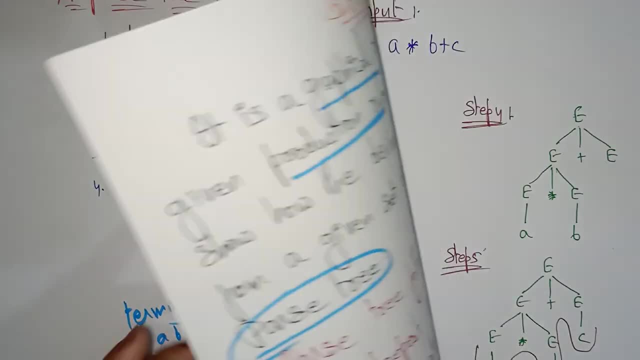 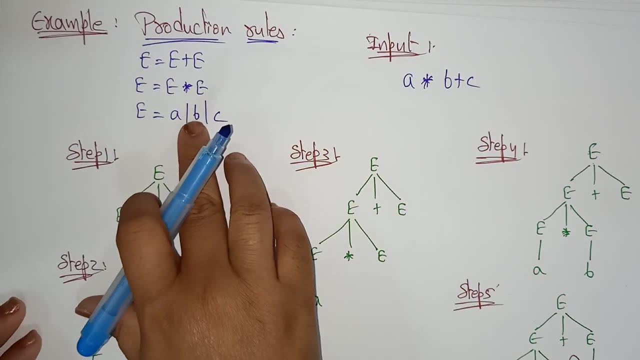 that are the non-terminals. so let me explain you one simple example about the derivation tree. so here i have taken some production rules. this is a production rule, okay, so e is equal to e, plus e is equal to e, into e is equal to a. e can be substituted with a or it can be substituted b. 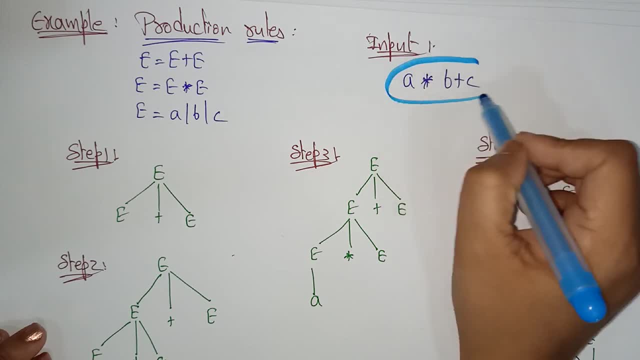 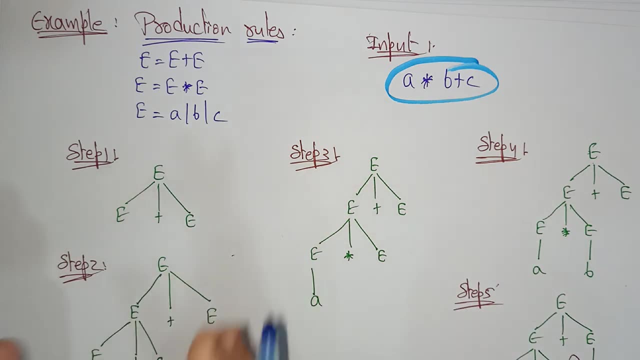 or it can substitute it with c and the input string that i need to be parsed is a star b plus c. okay, so what are the steps that we, if you want, you can go for the step by step or you can directly implement. okay, if you want you. 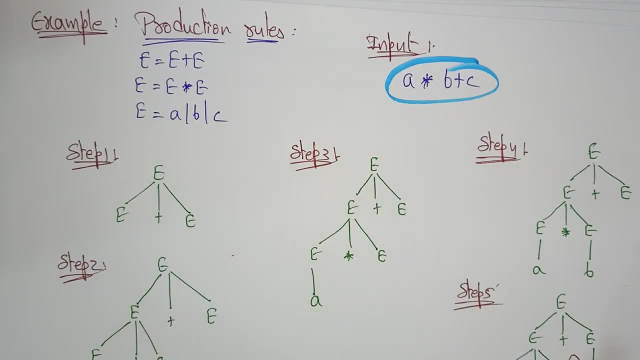 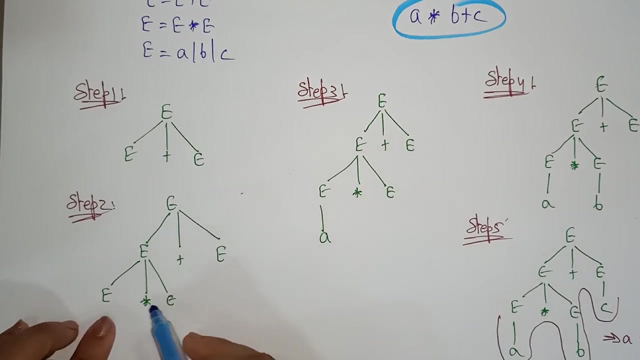 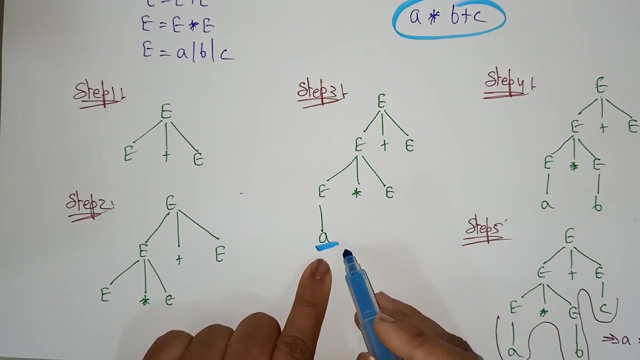 can directly uh go for the step five directly. okay, so starts with e. the e can be substituted with e, derives the e plus e, so e plus e. and step two: again, the e can be uh represented at e star e and this plus e. third step: again, this e can be replaced with the terminal a.